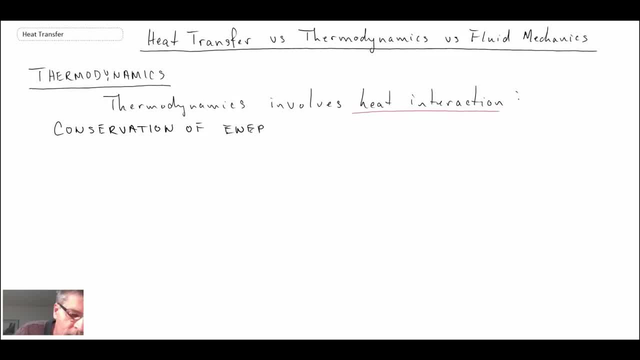 You could have either a closed system or an open system And, depending upon the system that you're using, the conservation of energy or the first law of thermodynamics will look a little different. Let's take a look at a closed system to begin with. 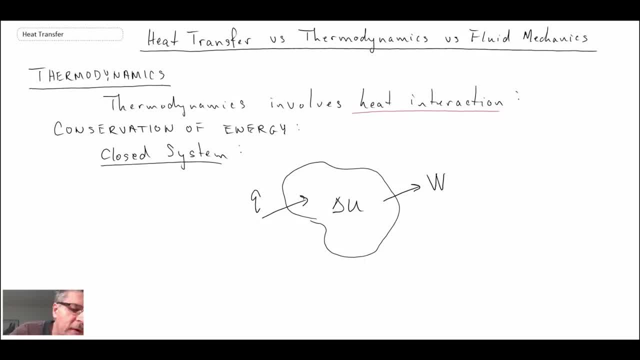 So when we're dealing with closed systems in thermodynamics, quite often what we will show is a closed system or a closed system. So an open system is the place on which it's interaction between the system and the surroundings, and interactions can be in the form of heat transfer, Q and, and I should point out, and I'll make a comment- 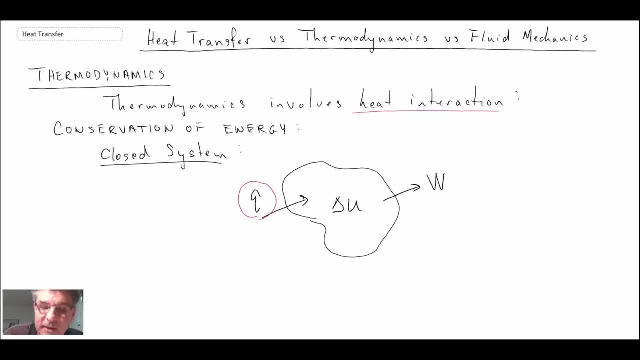 in a moment I'm using heat transfers designation for Q, so if you think this looks a little strange from a thermodynamics course, that's the reason. but what we have is we have heat interaction, we have work interaction and we have a change in the state and in this case we're looking at internal. 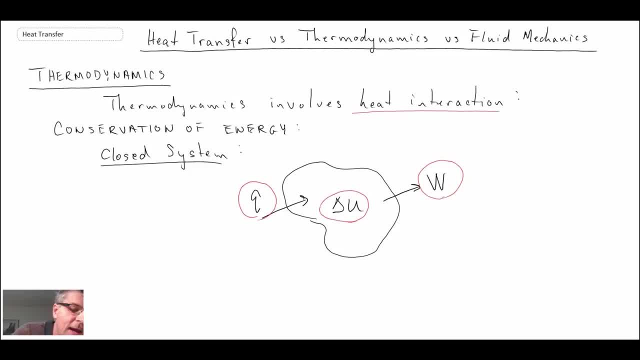 energy of our fixed mass system, and it usually when we write out the first law. so if we're writing out the first law for this type of system, it would look something like this: so what we have is we have heat transfer in minus work. in this case it is going. 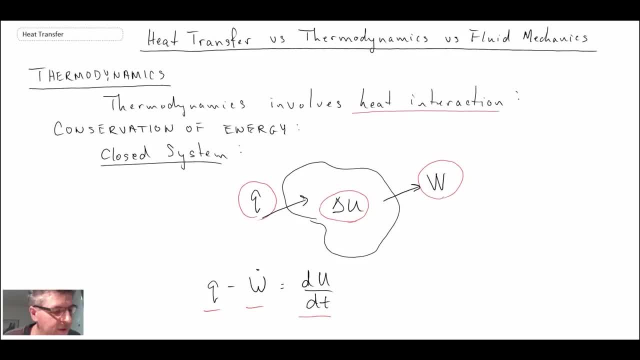 out is equal to the change in internal energy per unit time. concerning the unit say, I need to make a little bit of a comment here about the units that we're going to use and if you recall from thermodynamics and what we'll do, we'll take a look at the units for heat transfer. so quite 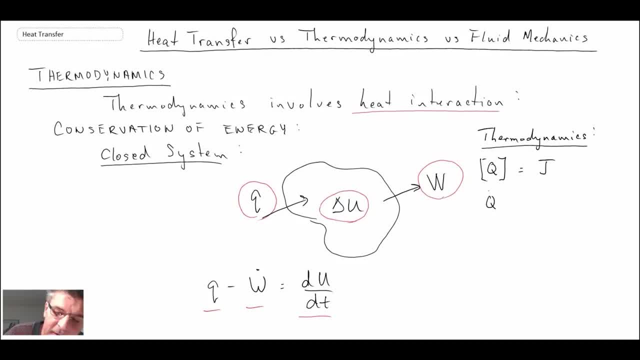 often will have capital Q. sometimes you'll see capital Q dot and that would denote joules per second. and then other times what we do is we divide by the mass flow rate, or m dot, and that gives us a little Q that we use in thermodynamics, and that's usually energy. 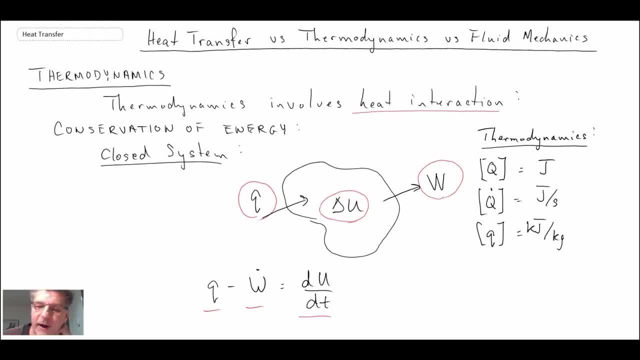 per unit mass, so I'll put kilojoules per kilogram, and that is what we've used in thermodynamics. now, when we're dealing with heat transfer, what we do, we use designation little queue, and that denotes joule per second or walked, and and so those will be the units that we use in heat transferring. 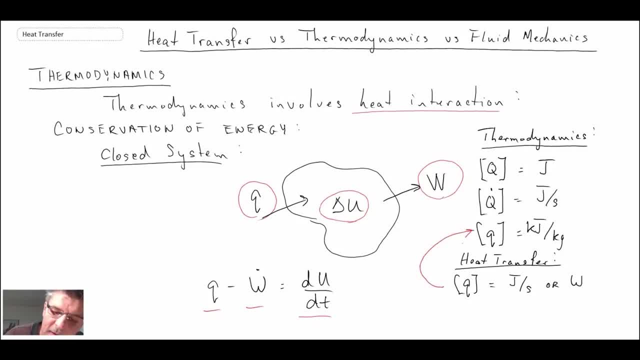 you notice by comparing these two together, they're different, and and so just don't get confused by that. in in heat transfer, little q denotes joules per second, and that's why this version of the first law might look a little funny or strange if you've just taken a course in thermodynamics or if you remember thermodynamics. 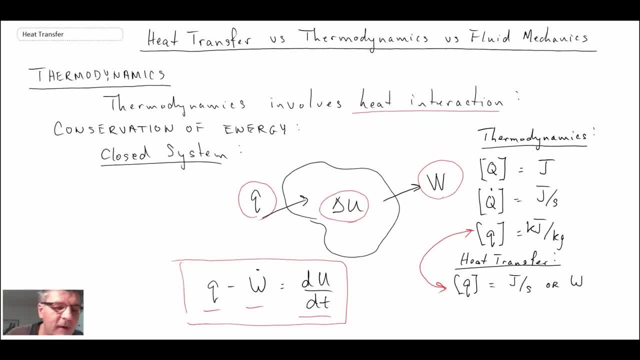 but that would be how heat transfer is involved in a closed system. so what we'd be doing in heat transfer is determining what this value of q would be. that usually when you're solving problems in thermodynamics, q is usually assumed or given and, if you recall, in thermal we also 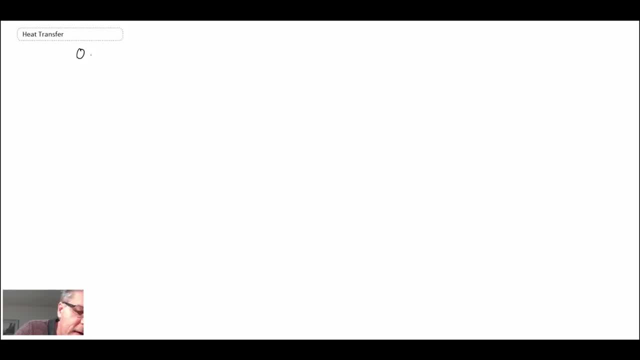 had systems where mass could be crossing our boundary, and those are open systems, and so what i'm going to do, i'm going to write out the what they sometimes call the fluid kidney. so it's just some system. there we have our system, we have mass crossing a couple of boundaries, we have an inlet and we have 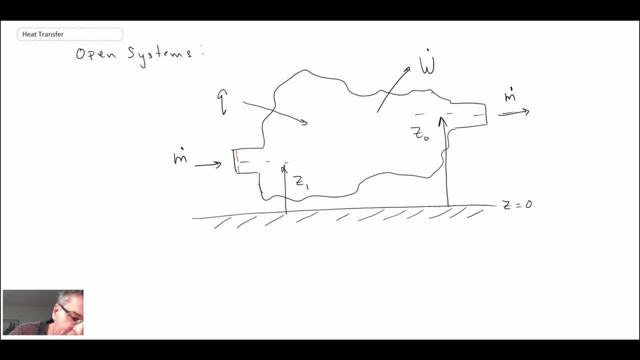 an exit and, given that we have mass crossing the boundaries, we have to be a little careful with the first law of thermodynamics, and we usually have information about the state coming in and the state leaving, and that is usually in the form of a little bit of information about where the 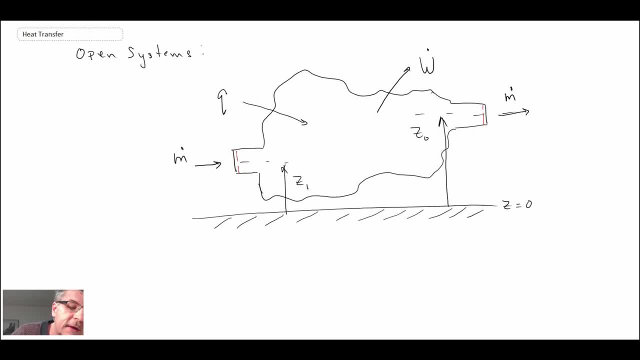 air and water line is coming and it's coming and out it's coming back, back and that's um of things such as the internal energy, little u uh pv, which is pressure times, the specific volume and the velocity, so that would be on inlet and then on exit. we would also know that information. 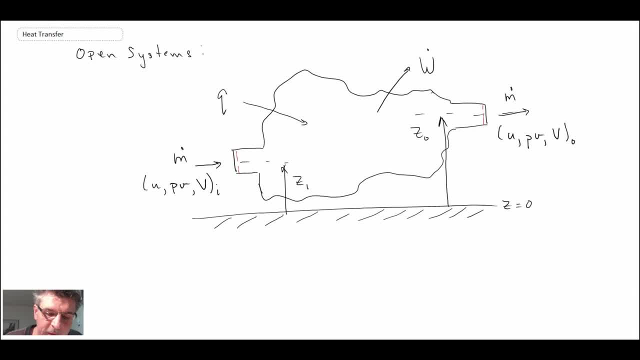 now we put this all together and that goes into the first law of thermodynamics. so, writing out the first law of thermodynamics for an open system, we have the following: okay, so there is our first law of thermodynamics. sometimes what we'll do is we'll cluster this into the enthalpy, and this is our kinetic energy and this is our potential. 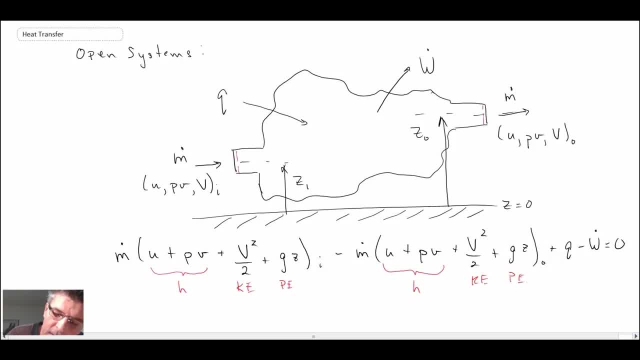 energy and we have mass flow rate coming and multiplying as a pre-multiplier and both the inlet and the outlet, and then we also have our heat transfer. we have our work. so in in this course, we're going to be focused on again estimating what that heat transfer might be, and that is again. 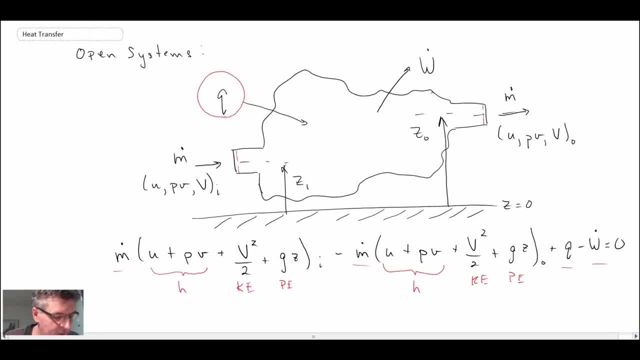 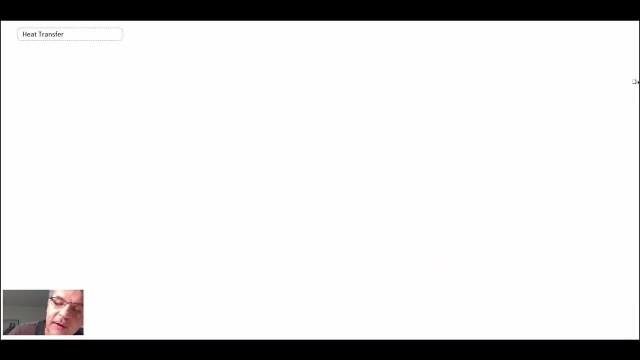 something that is quite often assumed or just given when we're doing thermodynamic calculations. so that is an open system in thermodynamics and where we see places where heat transfer comes in. and i just want to make a comment about thermodynamics. i'm going to write that out next. 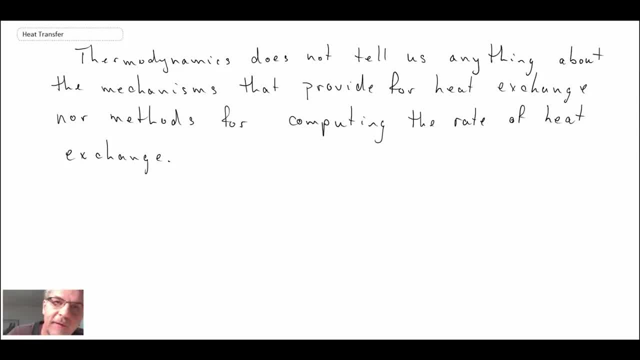 so when we're studying thermodynamics, as i mentioned, quite often, the heat transfer is given, and so thermodynamics tells us nothing about the mechanisms that the heat exchange is taking place under, nor does it provide methods for computing the rate of heat exchange. now, sometimes you'll give it a problem where you can actually calculate. 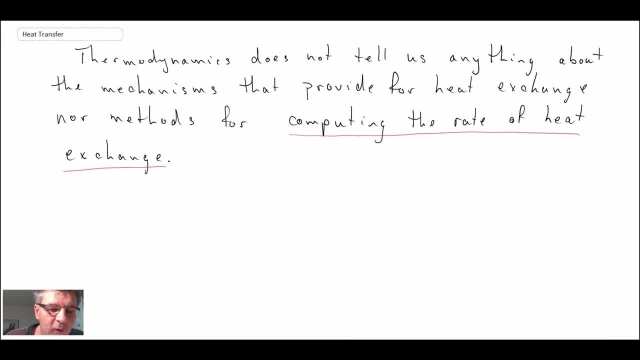 q that might be for a particular system, but you have no method of actually going in and calculating what that heat transfer would be for uh, given scenarios, and and so that's what we're going to be doing in this course, where we're going to be looking at the mechanisms. 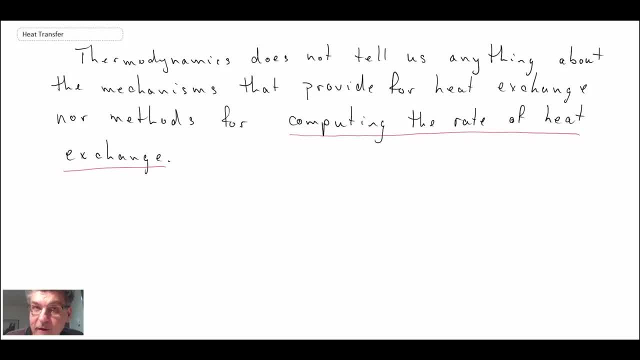 of heat transfer and we will be estimating the values of the heat transfer and with that, you're better equipped to be able to go in and then analyze systems, uh, be it with thermal dynamics or fluid mechanics, which we'll get to in a moment, but what we're going to do, let's take a. 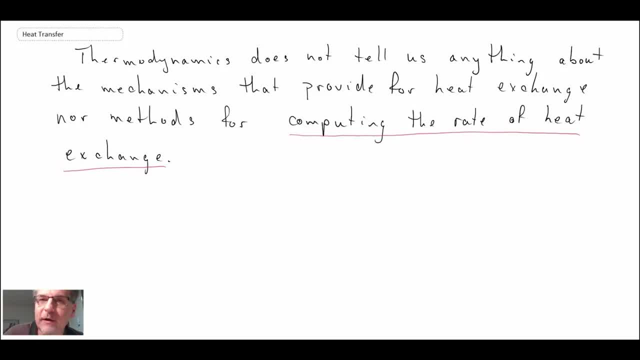 look at a brief example that kind of illustrates this and what we'll do. we're going to look at the case of throwing an iron ingot that is being quenched in oil. so there we have our problem statement. you look at any thermodynamics book under closed systems, fixed mass and guaranteed 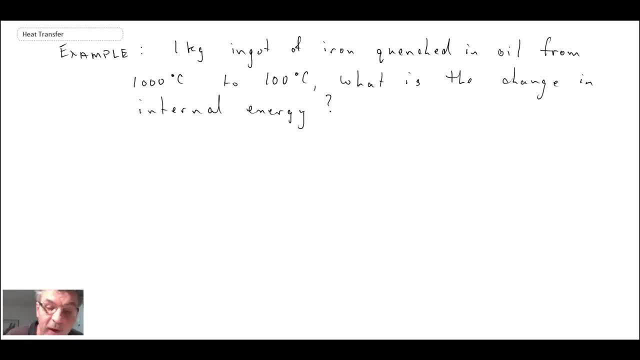 you'll find questions that look like this, and So, in order to solve this, what we want to do, we want to find what is the change in internal energy for an iron ingot that is quenched in oil and is going from 1000 degrees. 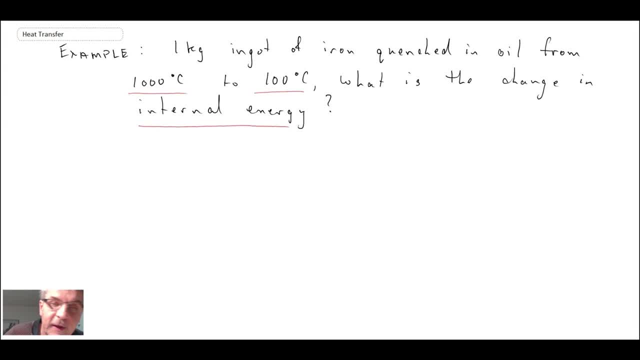 C down to 100 degrees C. So if you're doing thermal, what you do is you would go and you would find: well, we have to get the specific heat And, if you recall, du is Cvdt, so that is a way to evaluate the change in internal energy. 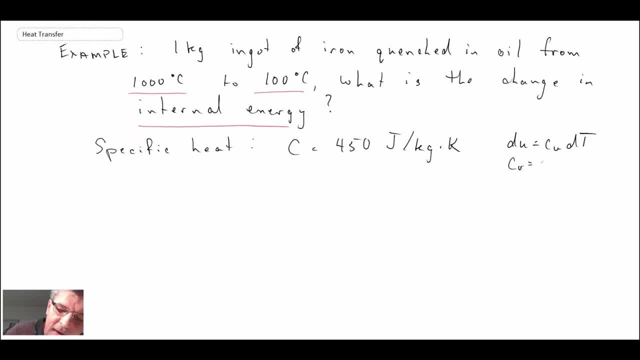 Now we're dealing with a solid and consequently Cv equals Cp, and so we don't really have to worry about that that. but we then go in and we evaluate the change in internal energy And we can plug in the values. Okay, so that's pretty. 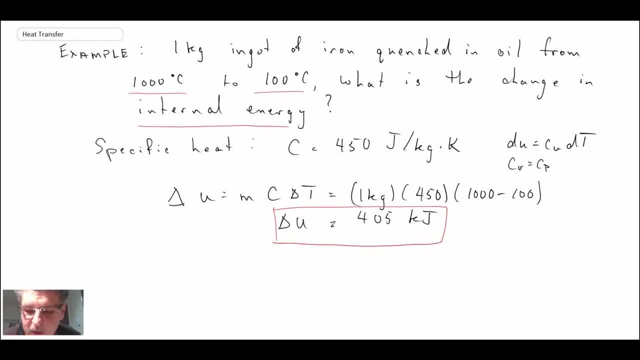 typical of something that you'll see in thermodynamics. You evaluate 405 kilojoules. Everything seems great. You've solved the problem. However, there are some other questions you may ask. Let's say, you want to know how long is this process going to take? Well, looking at, 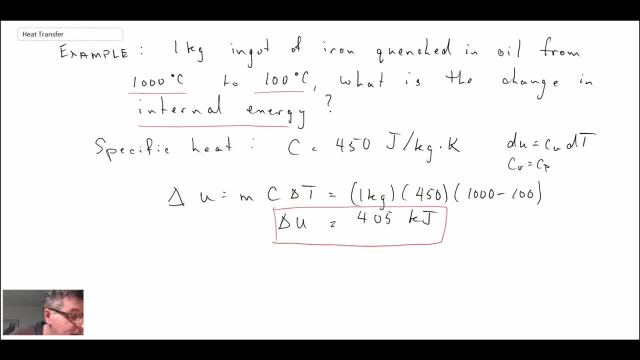 this. you have no idea, You have no way of being able to figure that out. Another thing: let's say we're dealing with ingot of iron quenched in oil. Let's say you're studying material science and you want to understand. 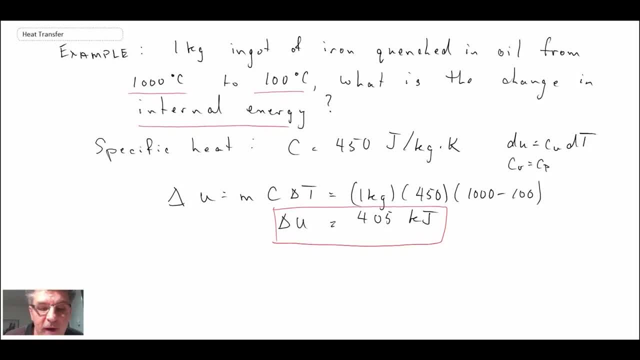 what the microstructure is Like on the inside of this ingot as it's going through this quenching process. So that means that you want to know what is the temperature distribution inside of this iron ingot and how is it going to change with time? Well, with 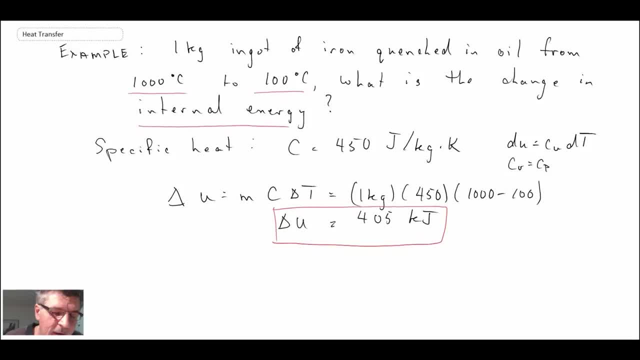 thermodynamics. you cannot figure that out, And so what we need to do, we need heat transfer in order to figure those things out. Now, with heat transfer, we'd be able to figure out the convective heat transfer coefficient on the outside. That would help. 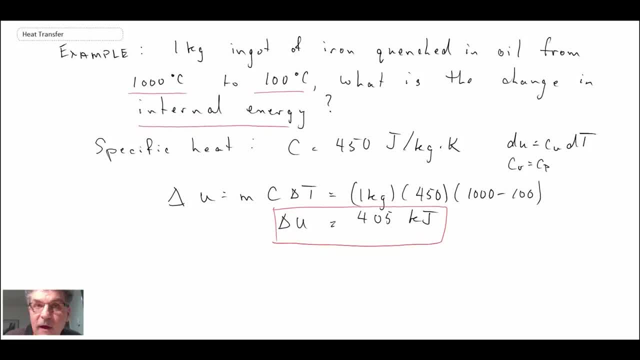 us figure out how long it's going to take, And we would also use conduction and the heat diffusion equation that we'll be looking at in this course to figure out how the temperature on the inside of this iron ingot is going to change as a function of time. So the questions: 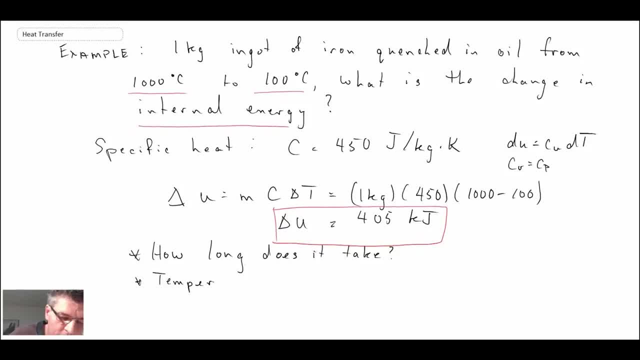 that we might ask, So you might want to know how long is it going to take? and temperature distribution, Heat transfer gives us these answers, And so that's why you're studying and watching this video, hopefully- and we'll watch more videos- And that way you'll be able to figure out how to solve this using. 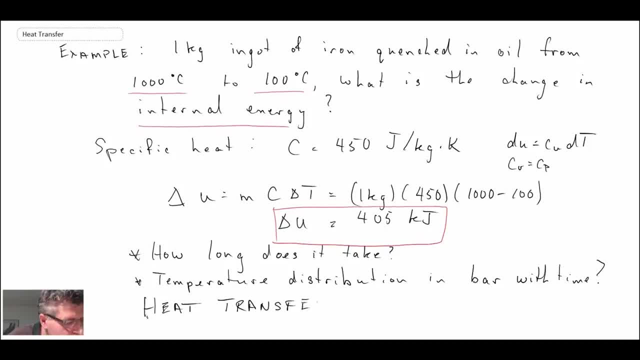 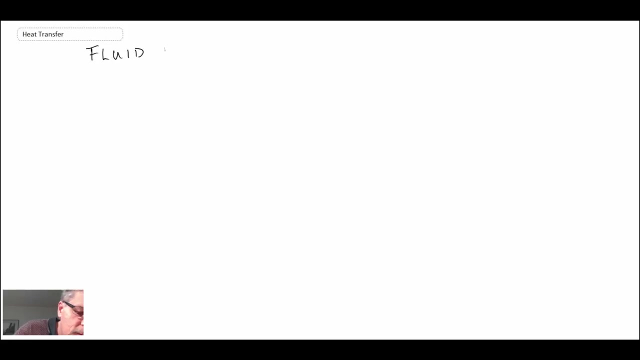 heat transfer. And if you're not interested in that and you just want the thermodynamic approach, go and watch the thermodynamics course. Okay, so that's thermodynamics. Let's take a look next at fluid mechanics. Okay, And the place where fluid mechanics comes in to heat transfer is when we have 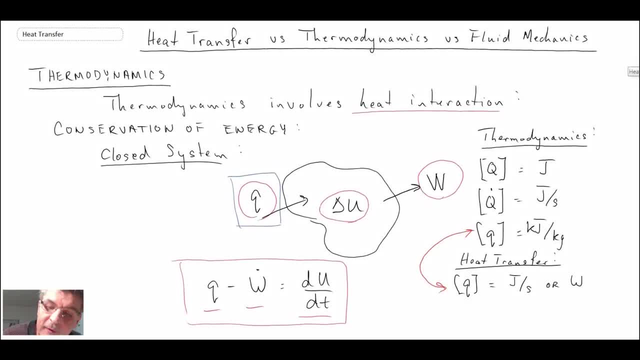 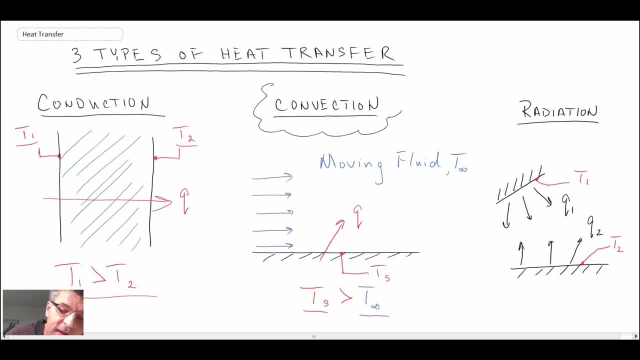 convective heat transfer. So let me scroll back here. This was from the previous lecture segment And what we did is we had convection here, So we looked at convection, convective heat transfer, We talked about that And you have a moving. 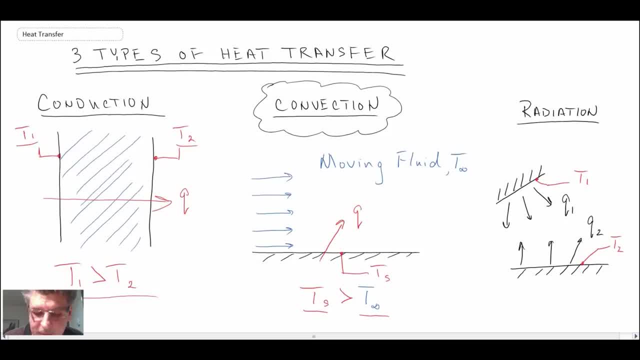 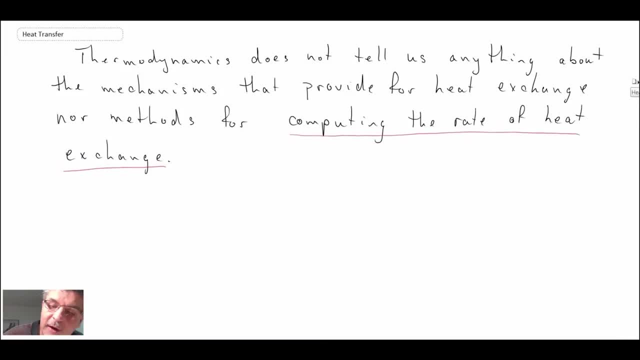 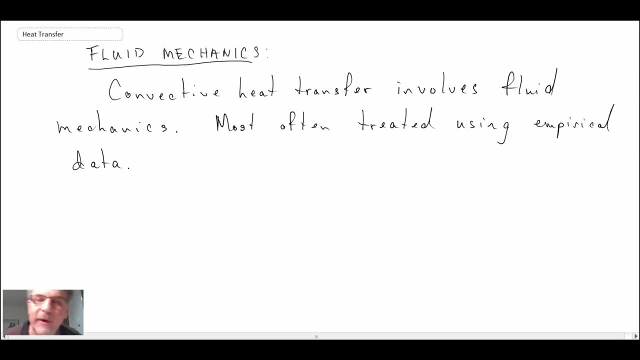 fluid coming over some surface. Here I draw it as being a really nice flat plate, But it could be any kind of irregular surface. So that is the place where fluid mechanics comes in to heat transfer. So what we'll be doing in this class, we'll be taking a look at convection.